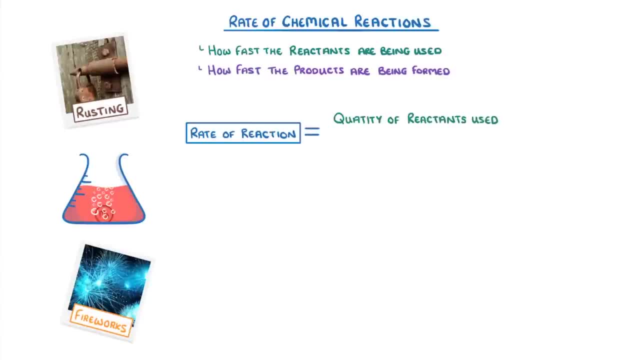 reaction is equal to the quantity of reactants used over the time it took for that change to occur, or that the rate of reaction is equal to the quantity of products formed over the time taken, With the quantities measured in grams or cm3, and time in seconds. For example, if 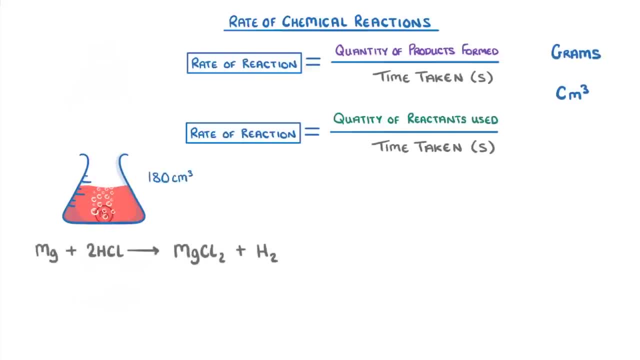 we knew that our magnesium and acid reaction produced 180 cm3 of hydrogen in 2 minutes, then, because hydrogen is a product, we would use our product form of the equation and do 180 cm3 divided by 120 seconds, because, remember, we have to convert our 2 minutes. 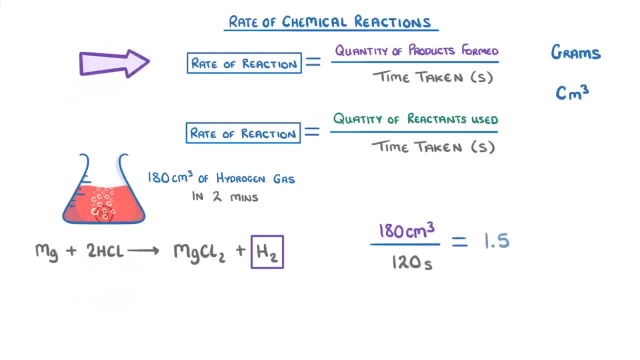 into seconds, which would give us a rate of 1.5 cm3 per second. Alternatively, if we had used 3 grams of magnesium and were told that it took 4 minutes to disappear completely and get used up, then we could use the other equation and do 3 grams divided. 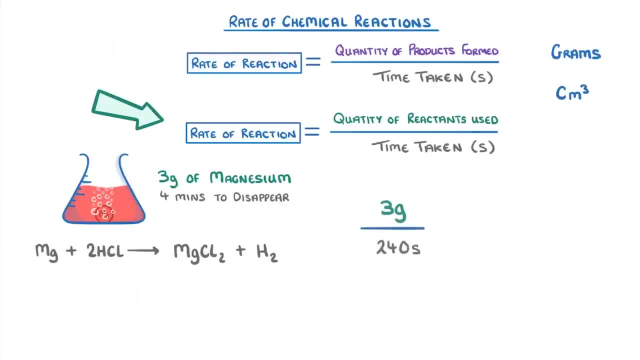 by 4 times 60, so 240 seconds, which gives us 0.0125 grams. Now these rates of reactions that we've calculated so far are actually the average or mean rates of reaction throughout the entire reaction. In reality, the rate would 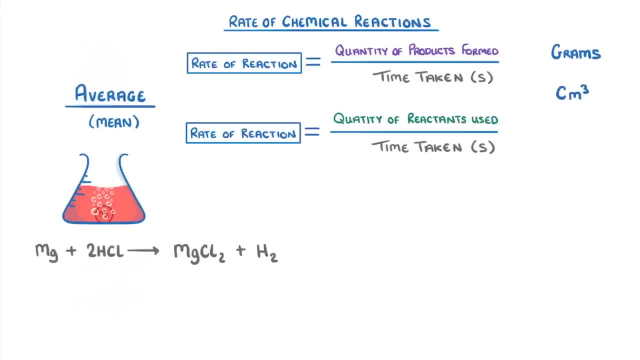 start off really fast when there are loads of reactants that can react together and then slow down as the reaction progresses and the reactants get used up. We can actually see how this works by plotting some graphs With time on the x-axis we can. 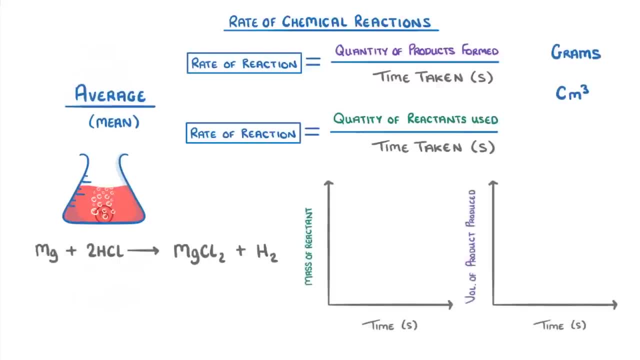 see that we have either mass of reactant remaining or volume of product produced on the y-axis. So on our left graph here, if we started with 3 grams of magnesium, then the mass of our reactant would start at 3 grams and at first fall quite rapidly, but then it would slow. 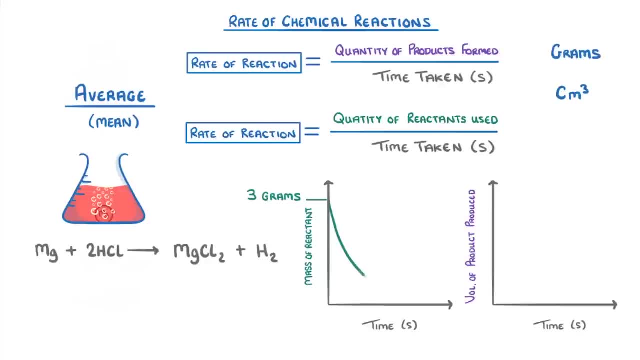 as the reaction progresses and it gets used up less quickly. Meanwhile, for our other graph, we know that at the beginning of the reaction we have no products, so it starts at zero. However, it very quickly increases as lots of hydrogen is produced at the beginning of.